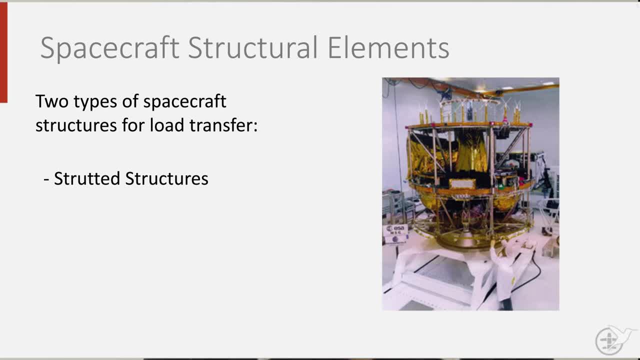 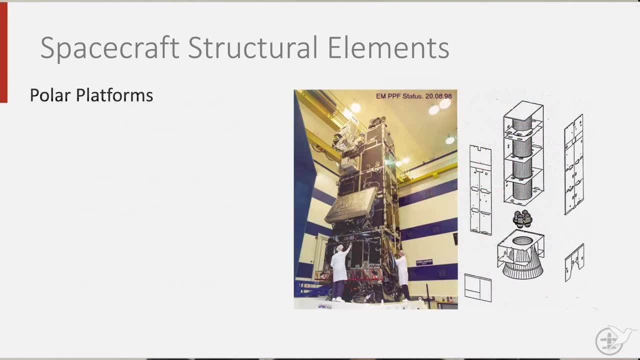 structures which are often three-dimensional trusses optimised for carrying loads, as can be seen here, or cylindrical sail structures, also known as polar platforms. Polar platforms are characterised by a central load-bearing member, such as a cone or a cylinder. All 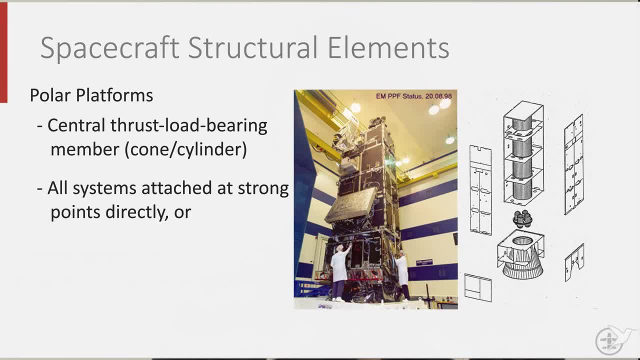 loads from the launch vehicle are transferred through this cylinder, and all systems within the spacecraft, such as the measuring equipment, are attached to this cylinder, either directly at strong points or by means of struts, platforms and shear webs. An example of such a polar 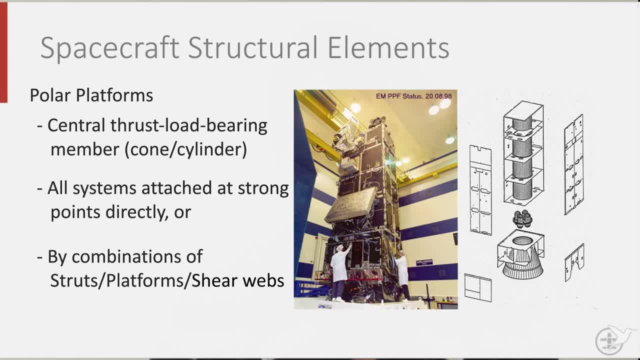 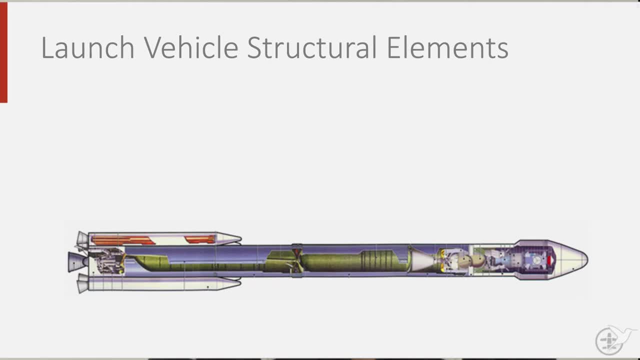 platform. spacecraft is the Envisat satellite which has a cylindrical shell, as you can see here. If we take a good look at a launch vehicle such as this one here, we can distinguish four main structural elements: The fairings, the stage structure, the thrust structure. 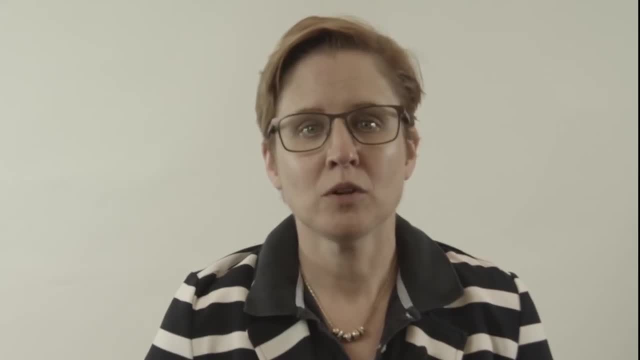 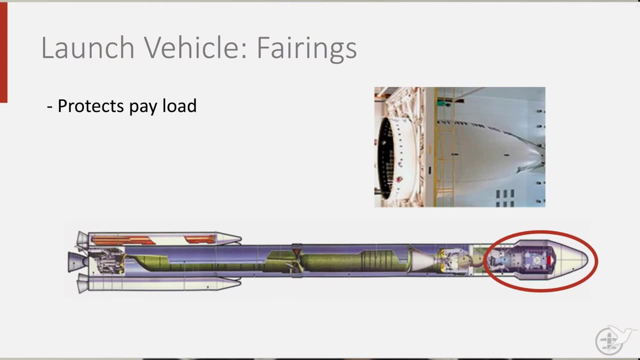 and the adapters. Let me discuss each element one by one, starting with the fairings. Fairings have as their main function to protect the payload during the launch from the aggressive environment around it. They must maintain their shape and are therefore often designed. 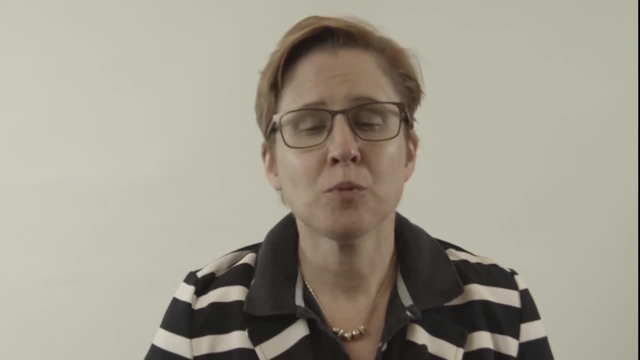 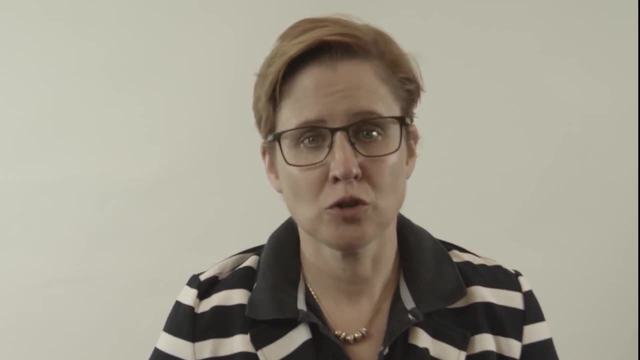 to protect the payload during the launch. The stage structures are the structures that form the body of the rocket. A rocket often has multiple stages, each with their own propulsion system, so it can dispose of used stages during the launch, eliminating weight and increasing acceleration. There are two types of space structures: One where 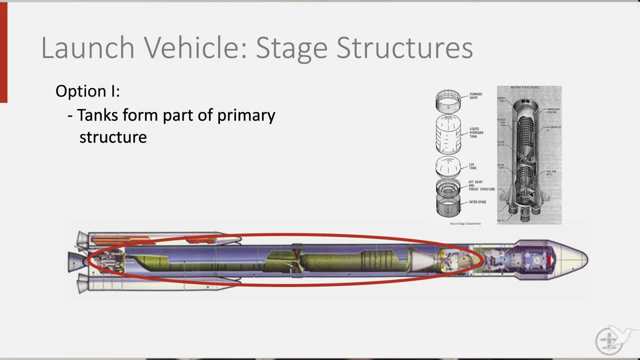 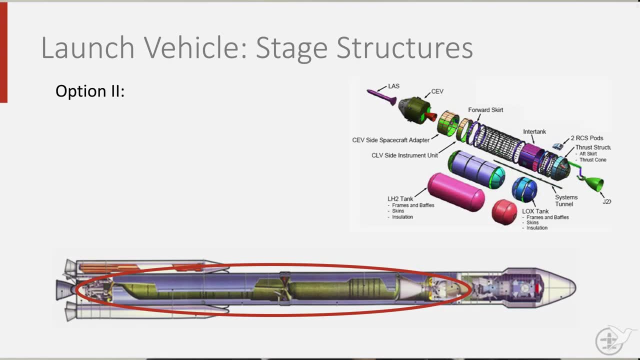 fuel tanks are part of the primary load-carrying structure, such as the Saturn V rocket. These structures resemble a semi-monocoque structure with internal stiffeners. A second option is a separate tank which is not part of the primary structure. 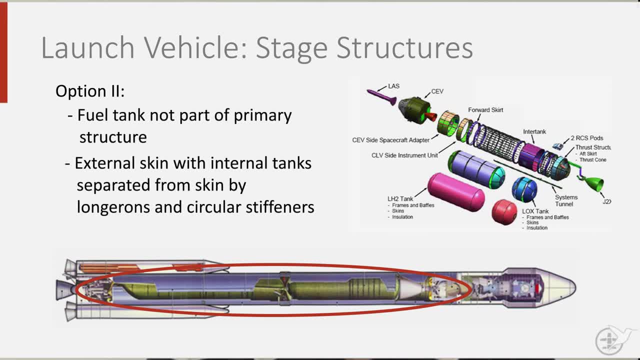 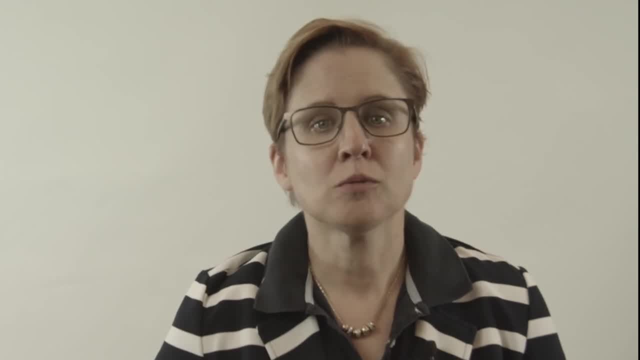 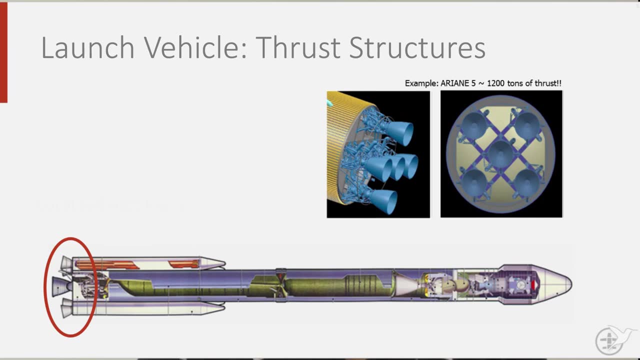 There is an external skin with the internal tanks separated from the skin by longer rods and circular stiffeners. The infamous V2 rocket had such a structure. Thrust structures transfer the enormous thrust from the engines to the main stages of the launcher. To put a number on it, the European Ariane 5 rocket produces 15,000 kN at liftoff. 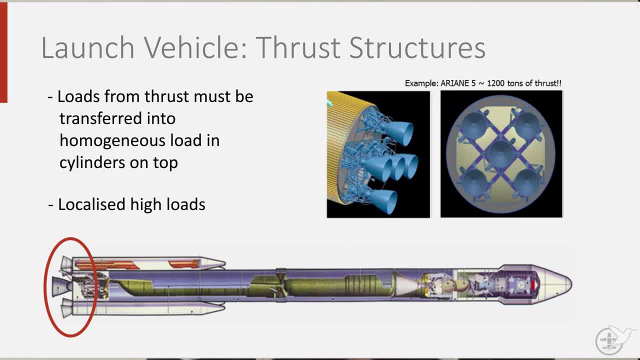 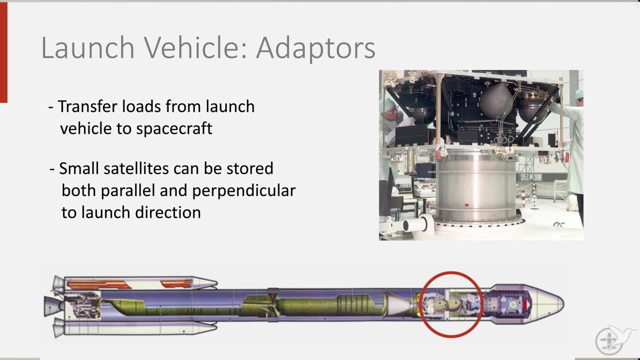 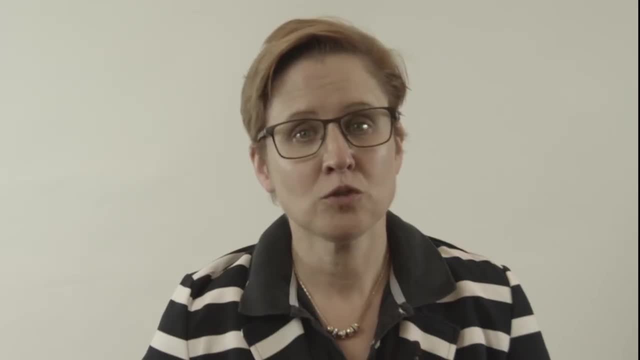 This concentrated load must be distributed into the stage structure via a conical structure. Finally, the adapters. They transfer the loads from the launch vehicle to the spacecraft. Here you see the adapter for the European Hipparcos satellite. Space is definitely aviation's big brother when it comes to structures. This makes spacecraft and launch. 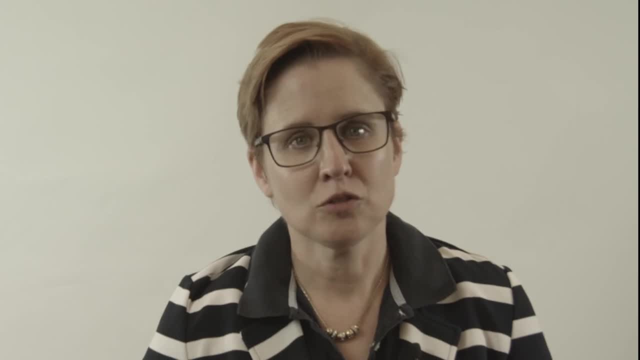 vehicle design a complex and challenging enterprise and has not yet reached its final frontier.